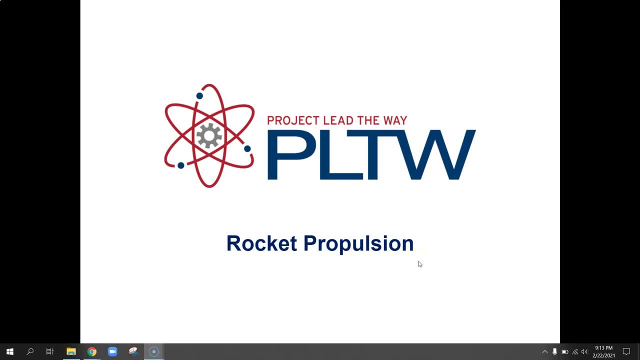 All right, everybody, this video covers rocket propulsion. Obviously, as the slide tells you, it's 2.2.4, modified in the Mr T way, so this won't exactly match what you would download from my PLTW, But it's pretty close. I think it's a little bit more explanatory. So it's going to cover some equations and some concepts that we're going to use, that you're going to use, to design and build your own rocket. 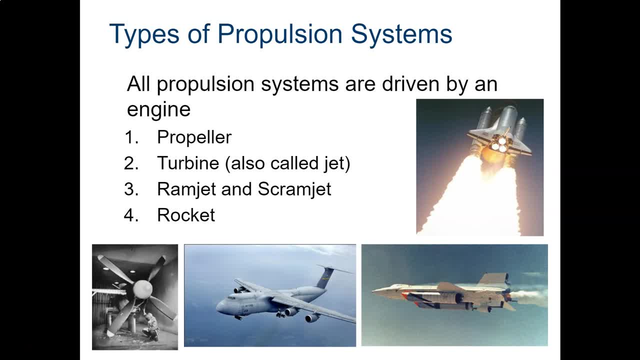 So just to recall- we're still on the topic of propulsion- We've talked a little bit about propellers. So remember, a propeller is just a rotating wing that, instead of lift when you turn it 90 degrees, it creates thrust. 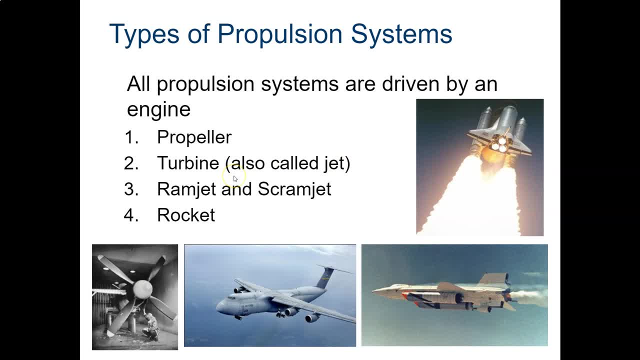 We know all about turbines. We've talked a little bit about ramjets, And, if you don't remember, a scramjet is a supersonic combustion ramjet. And so the fourth thing, the last thing to really cover on the topic of propulsion are rockets. 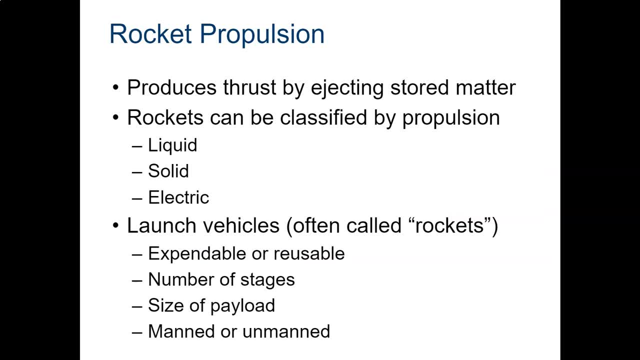 So a rocket produces thrust by ejecting stored matter and also a change in pressure. They can be classified by liquid, solid or oxygene, Electric- Mostly liquid and solid is what you're familiar with. Electric engines are used in the vacuum of space. 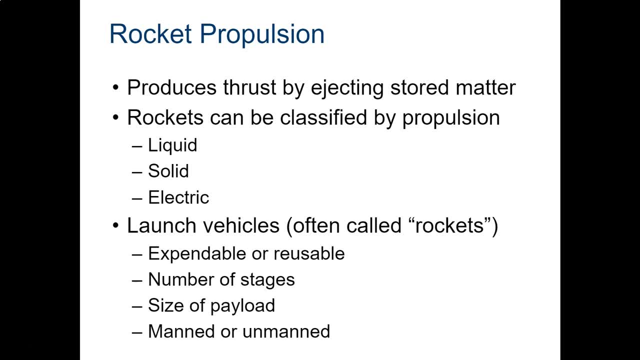 One thing that's a little bit different here is what I call launch vehicles. If you look at the PLTW slides it's a little bit confusing. So the term or the word rockets is often used interchangeably, So it can mean the rocket engine itself. 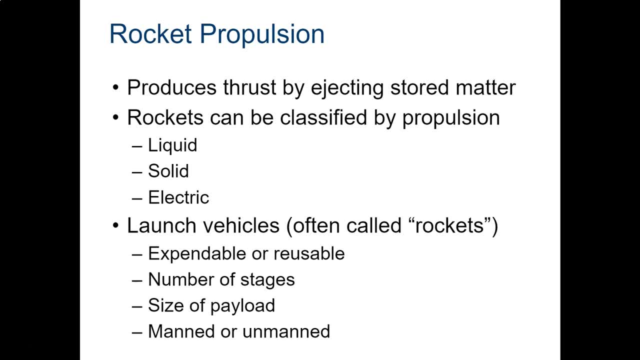 Some people say rocket motor, but it can also mean a launch vehicle. So a launch vehicle would be like the Space Shuttle or the Saturn V that sent the Apollo astronauts to the moon, And you can look at those in a number of different ways as well. 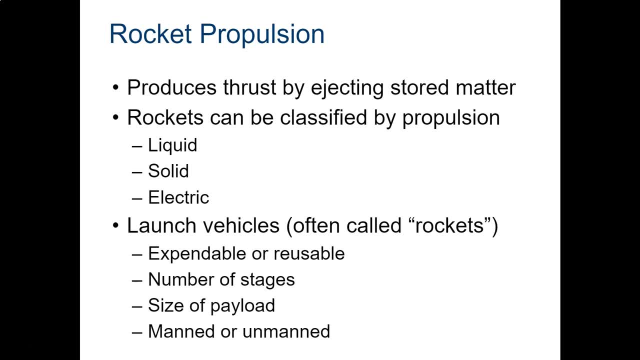 So there's expendable or reusable. For example, SpaceX has reusable rockets. The solid rocket boosters for the Space Shuttle were also reusable. You can talk about the number of stages- There are multiple stages- the kind and size of the payload and if it's manned or unmanned. 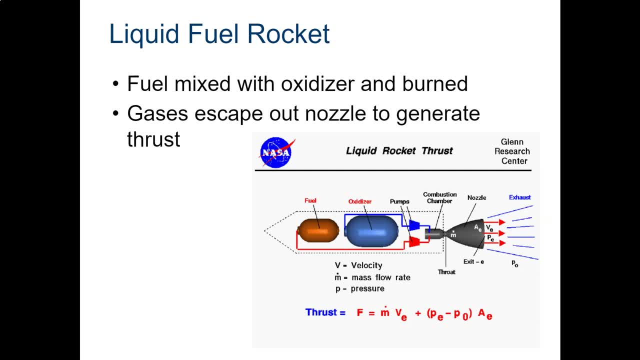 So let's take a look at a liquid rocket And they all kind of work the same way. I'm just going to kind of ignore these bullets up here for now. But in the liquid rocket you have a fuel and an oxidizer. 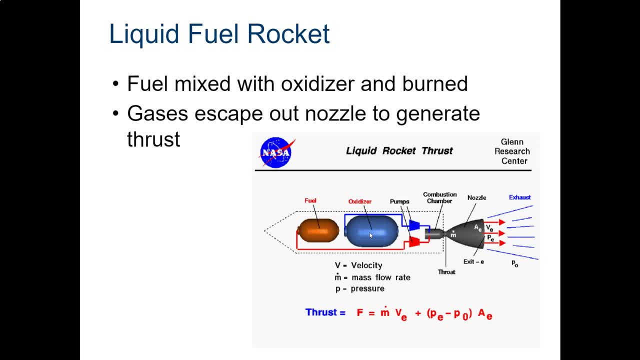 They can be different. It's common to have hydrogen for a fuel and oxygen for an oxidizer. They mix in the combustion chamber here And some of the terminology that you need to know are things like combustion chamber, throat. That's where things converge. 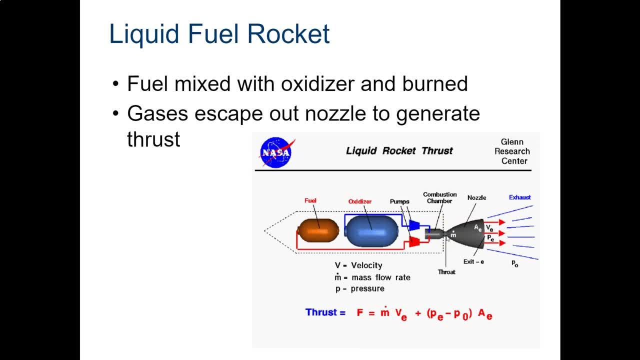 That's the smallest area- And we'll learn a little bit about that in an upcoming slide- Smallest area in the rocket engine itself and then the nozzle where all the gases are expelled. So this is the exit and you can see we associate some things with the exit. So there's. 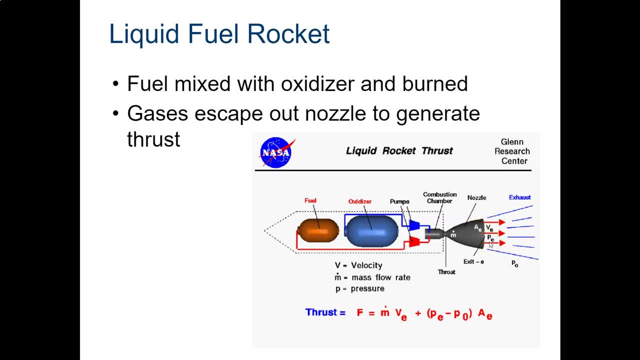 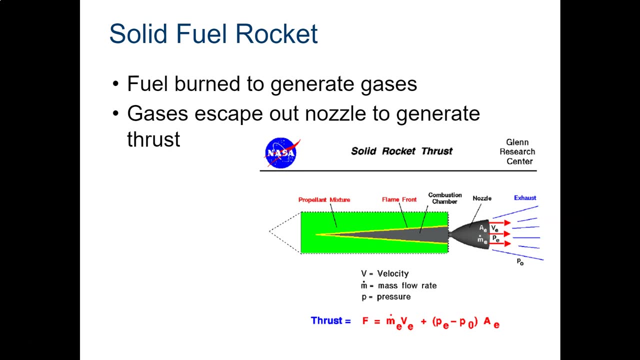 the area, the velocity, the pressure at the exit and then P sub zero is the free stream pressure. A solid rocket motor or solid fuel rocket? it does the same thing. It ejects hot gas in a very fast manner, but it burns a mixture here, and a mixture totally depends on. 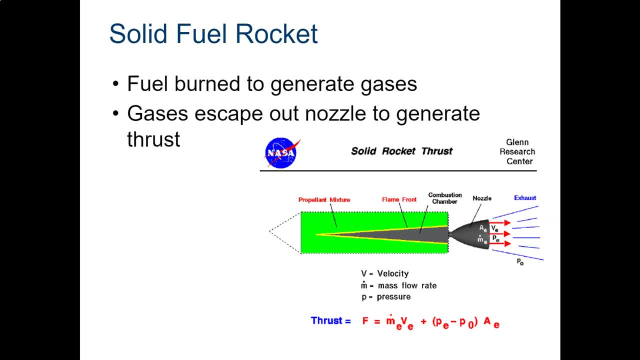 the mission- For example, the solid rocket motors for the space shuttle- uses a lot different mixture than what we will use. We're going to use some Estes motors. You can change what this mixture is. You can change the shape of the, of the. 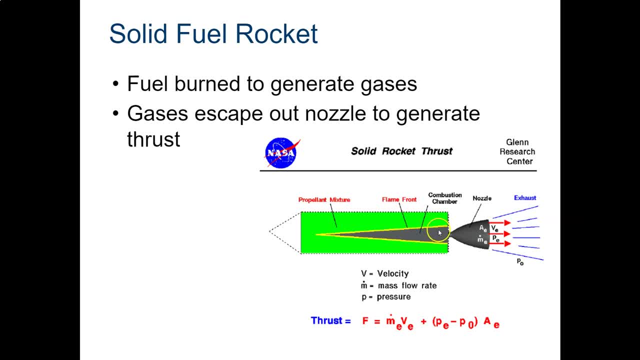 cross sectional area and that's going to change the thrust. So it starts burning down here towards the combustion chamber. This whole thing is really a combustion chamber, but it starts burning near the nozzle typically and will go from as our screen goes, from right to left Once you start. 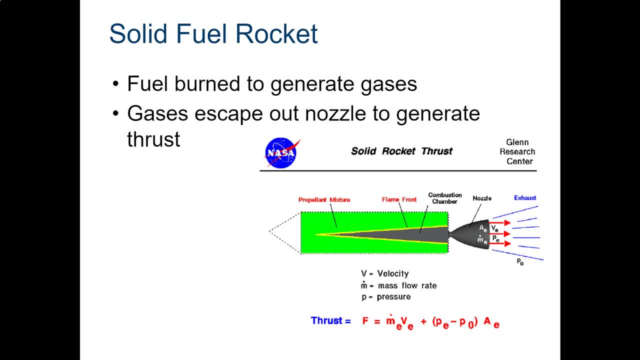 burning this, a solid rocket motor, you cannot stop it, Unlike a liquid motor, you can turn off the fuel, You can turn off the oxygen, You can turn off the oxidizer. You can control that. A solid rocket motor you cannot. That's one big difference to know. 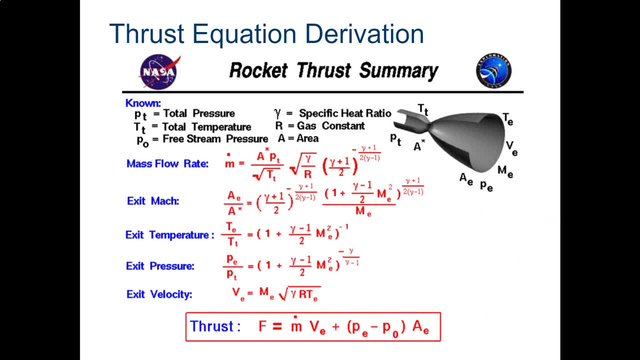 Here's some a really scary-looking I know. What I really want you to pay attention to is down at the bottom, and we'll get to that in a second. Just some definitions and some terminology. Here shows the basic bell shape. bell shape of a rocket engine. So here we have the combustion chamber up top and there are 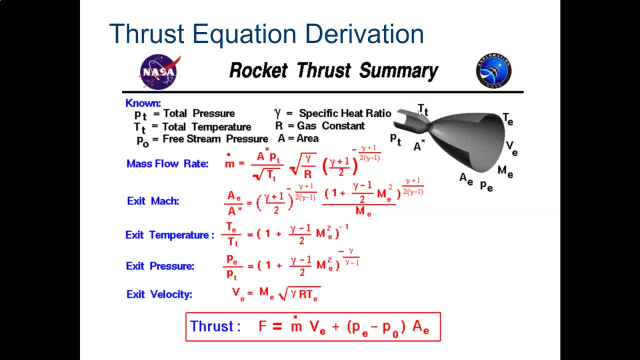 pressures and temperatures associated with almost everything in propulsion. So in the combustion chamber we call those total pressure and total temperature A star, and that's how you say it. A star is the area of the throat. We don't really talk about the area of the combustion chamber. 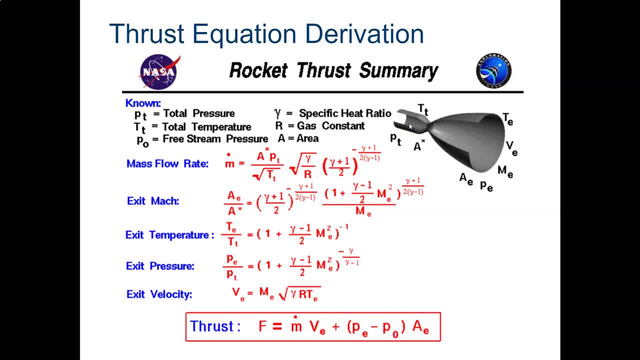 We characterize that by temperatures and pressures And then finally, you can see the nozzle and it expands, gets bigger, the area gets bigger because right at the throat, you want flow to be super or not supersonic. you want it to be sonic, You want the Mach number here. 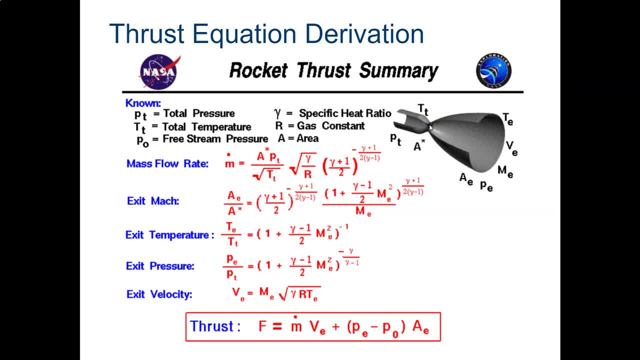 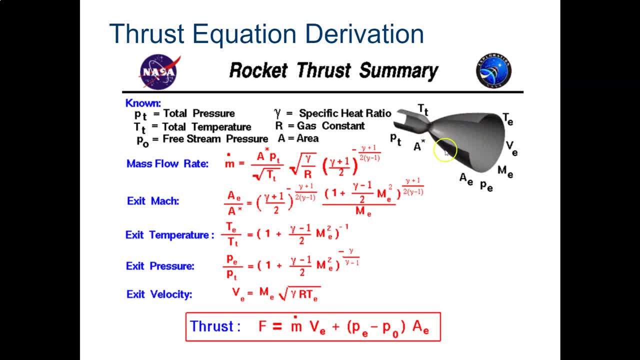 what happens is, though, in a rocket engine, and the reason you have this bell-shaped nozzle is once it reaches sonic conditions. here things flip, So it actually becomes faster and it gets. the Mach number here at the exit is greater than one. That's what you want in your. 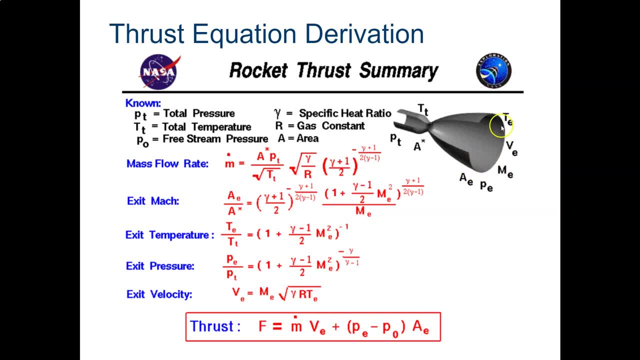 rocket engine. So we define some terms here. At the exit you can see temperature, velocity, Mach number, pressure and so on. So it gives you some other definitions. up here We can look at mass flow rate and it's really defined by the area of the throat, some combustion chamber temperatures and 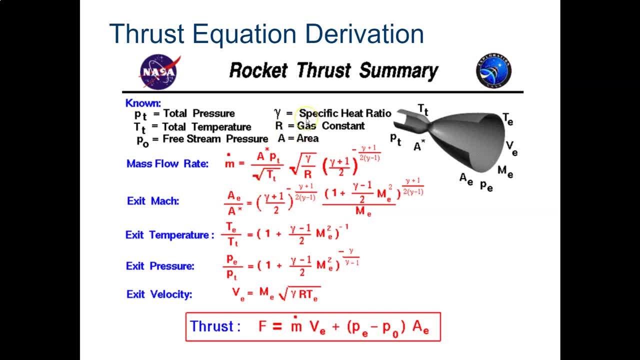 pressures and then the gas constant and specific heat ratios. You might remember that from chemistry That's totally dependent on the fuel and the oxidizer, So I'm not going to go through all of these equations. I don't expect you to know all these equations or even how they were derived. That's something that you'll get. 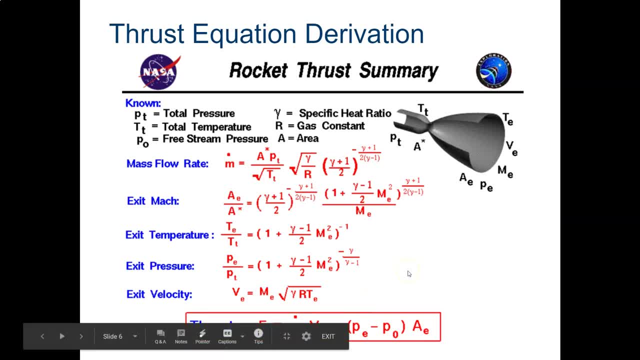 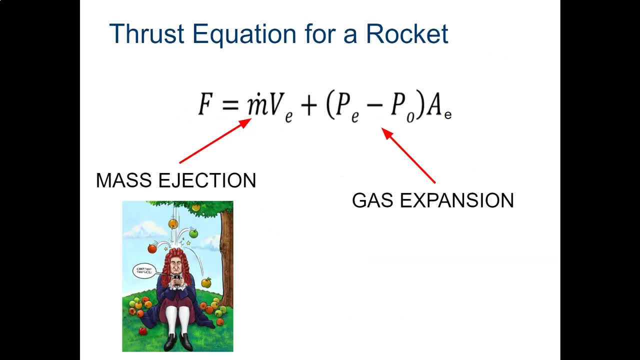 to in college. But let's take a look at the thrust equation. It has a couple of different terms. So let's go to the next slide and take a little closer look. So the two terms kind of look should look familiar to you. The first term is: 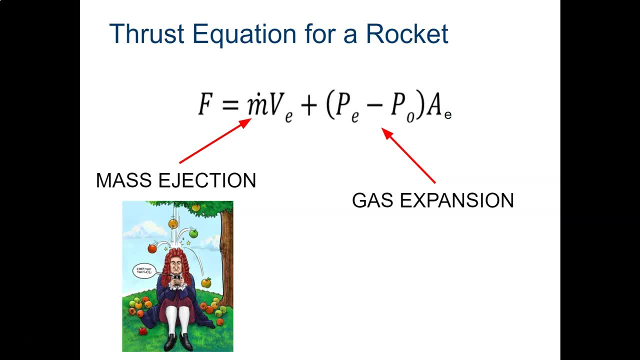 relating to the mass that's ejected. So it's not uncommon for a rocket, especially a large rocket, to lose 90 percent of its mass during launch. That's not going to happen in the rockets that we're going to launch, although they will lose mass because they burn fuel. And then the second. 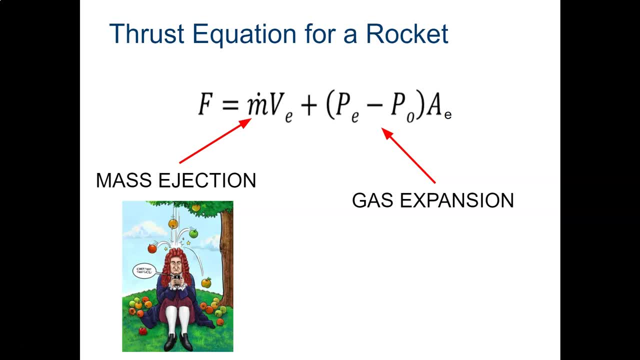 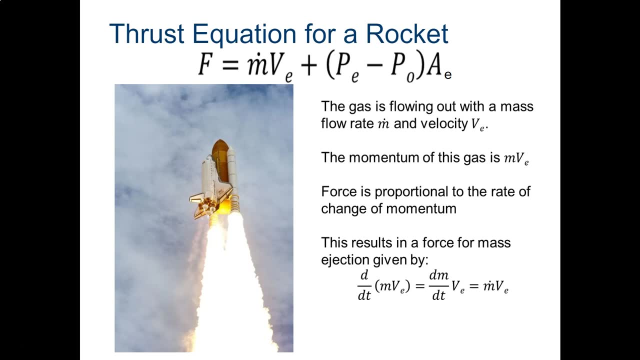 part has to do with gas expansion through the nozzle. So we take a look at that first term, m dot v. If we remember m dot and if you want to take a look down here at the bottom, it kind of explains that. 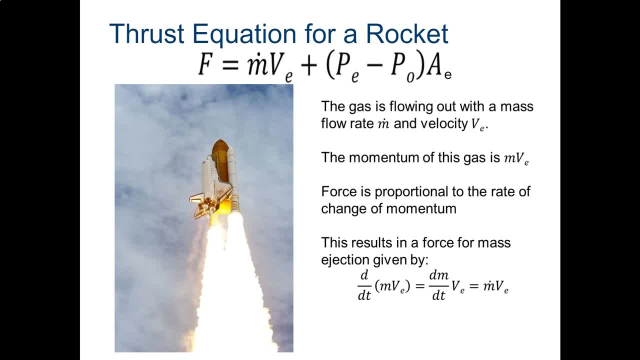 It's really a change in momentum is what this term is all about. So if we take m dot and we remember that that is mass per time and we just move the time underneath the v, velocity over time is really acceleration. So we have: force equals mass times, acceleration, Newton's second law. So that has to do. that term has to do. 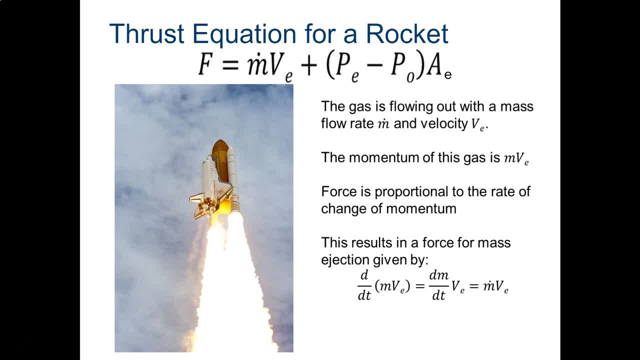 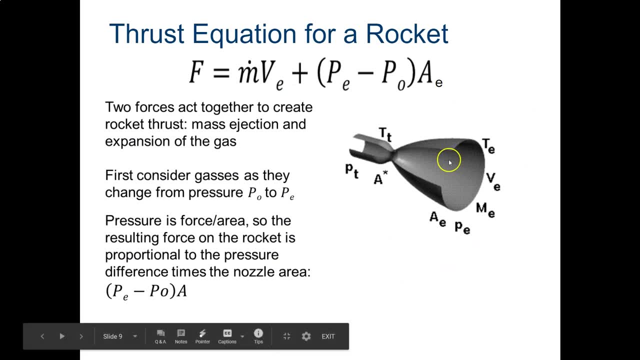 strictly with the mass that's being ejected. we have a. we get a force from that. and then the second term has to do with pressure differences. so remember, P naught or P zero is the free stream condition. so it's, it's the condition out here, whether it be the vacuum of space, in which case P naught would be close to, 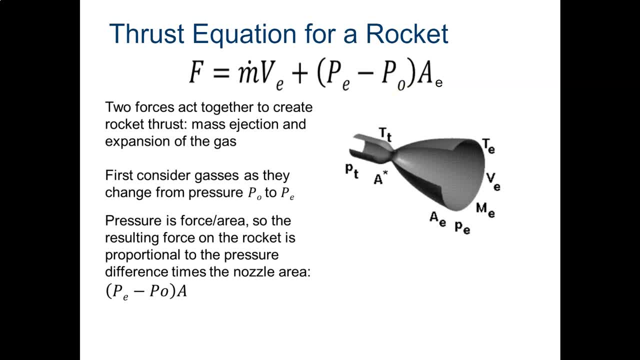 zero or close enough to be zero where we could ignore it, but that's not necessarily the case on the surface of the earth when you're launching a large rocket. so let's take a look at the units for pressure. remember, the units for pressure are a force per area, force per unit area, so we take a force per area. 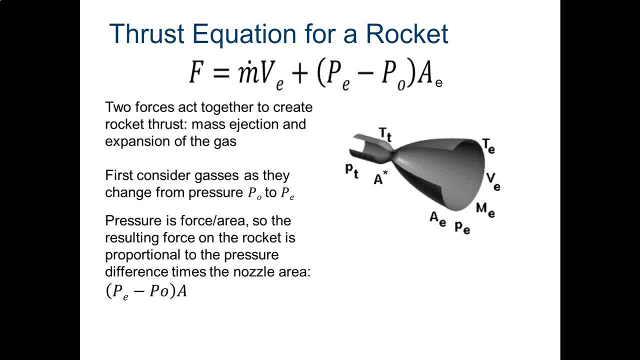 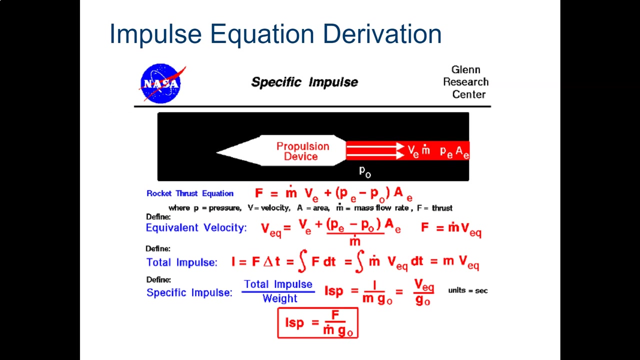 and we multiply it by an area, we get a force. so it's really just the exit pressure minus the atmospheric pressure you times area of the exit. we add those two things together. that's how we get the total rocket thrust couple more terms that you need to know and understand. so so let's start with 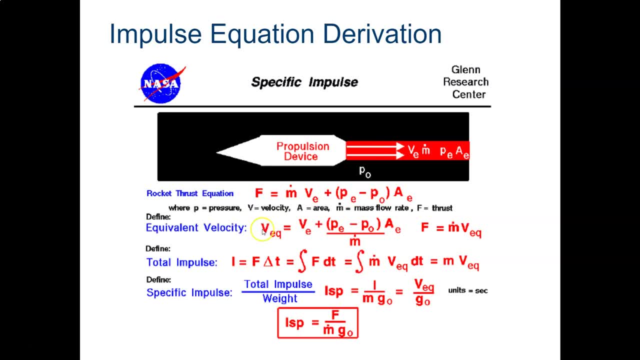 the rocket thrust equation that we just talked about. if we divide both terms by m dot, we can we end up with velocity. so there's exit velocity and then there's- we would associate with the pressure difference- and we call those two velocities, when we add them up, the equivalent velocity. I'm not going to. 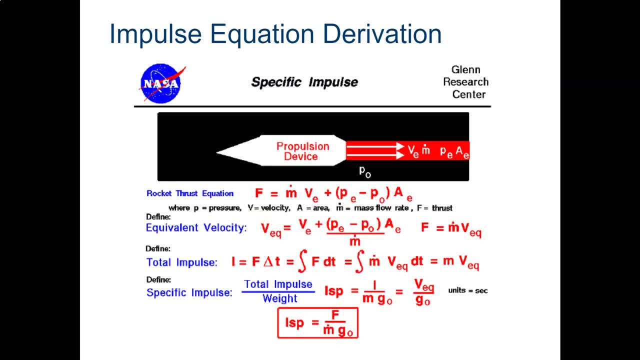 make you calculate anything with respect to equivalent velocity. maybe there might be a quiz someday on it, but not right now. one thing, two things I should say, rather, that I want you to understand. one is impulse. so impulse is a force times a time and it gives you some a derivation over here, using integration and some. 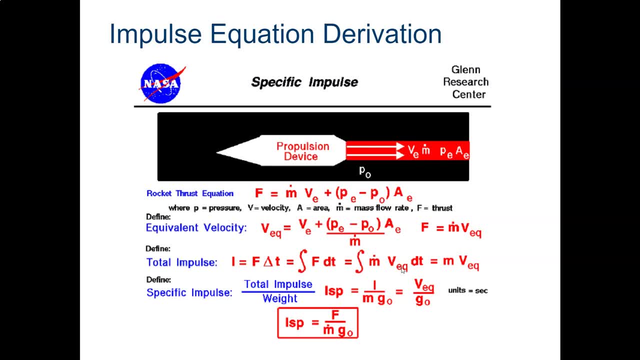 calculus. I know some of you aren't in calculus. some of you are in calc 3. I don't expect you to to know that if you know calc and you're comfortable with it and you understand this great, what I want you to understand is that impulse. 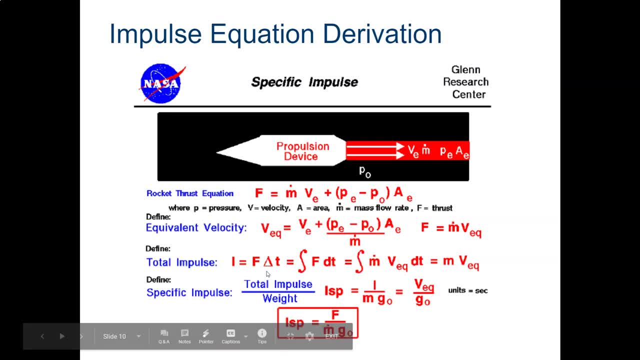 is a force times a time. that's something that we really need to look at and understand. in terms of rocket performance, you specific impulse is basically taking the total impulse and dividing by the weight, and it's called ISP, for that's supposed to be a subscript. they're. 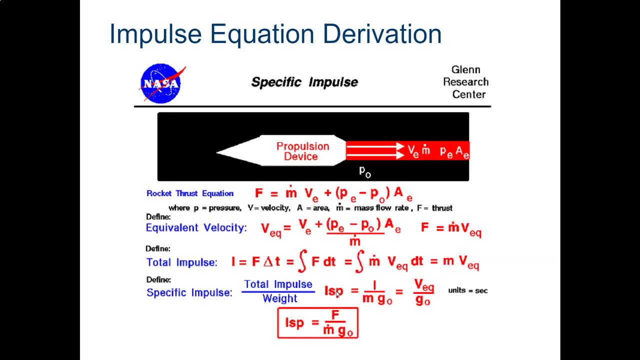 specific. it's called specific impulse and that is really mostly related to the propellant and it is a standard measure in industry of efficiency. so some common values would be two or three hundred, and the units which are really important here are seconds. what are the units for total? 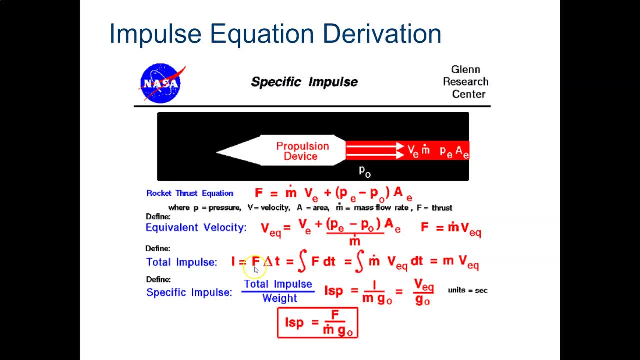 impulse. well, force would be pounds or Newton's times seconds, so it's usually pound seconds or Newton seconds for impulse. we're going to be working with some smaller model rocket engines, so we're going to use Newton seconds. but make sure that you know total impulse and specific impulse. 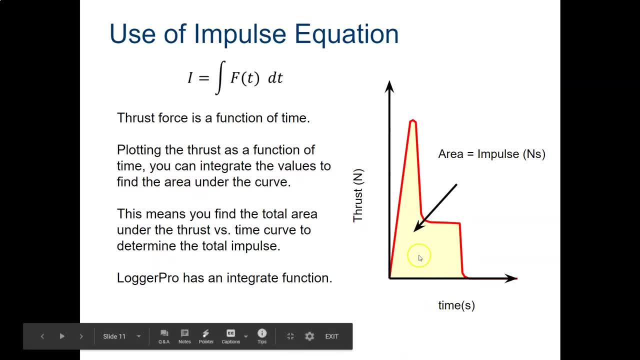 that you're measurement and a number Unto get some gains. so that's 2018. then give us about any of these numbers, but I'm going to start with just the optimize in. we would haveed a little bit of a plan which common teachers atory here is typically stilldin in, a little bit ev debe did might have done. 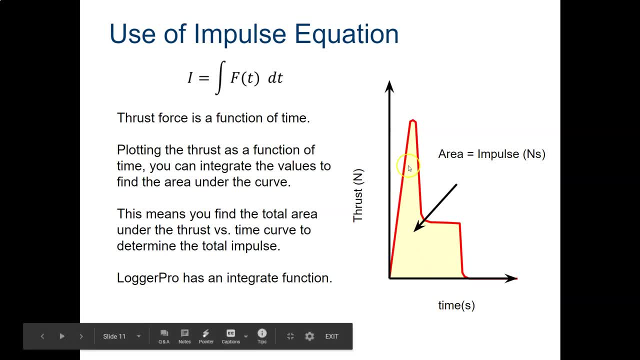 this in the last several years before I went very slowly. this image- it's a pretty good sample, but we are going to talk more about� circle of the curve. basic version is composed of more oder起來, using spans for chords and dynamically using the pulse of something else. so let's take a look at this. is what a typical thrust curve is called looks like for a model rocket like the SDS, and we will take a look at that on some upcoming slides as well. I'll take a closer look at this. but the total impulse is the area under the curve. so this red line is basically a map- it's a embassy craft- of the thrust of the engine mapped over time. 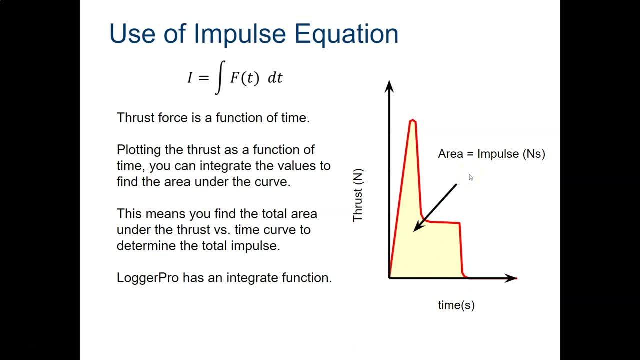 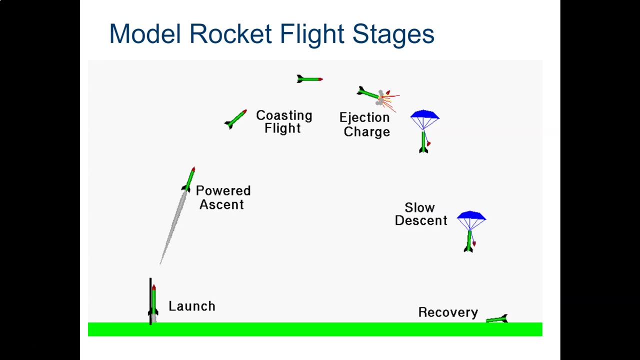 under that curve is a total impulse. that's something you need to know. we're going to work with some thrust curves, so you'll need to know that you're not going to have to do any integration. logger Pro will do it for you- model rocket flight stages and we're actually going to come back to this. I left this. 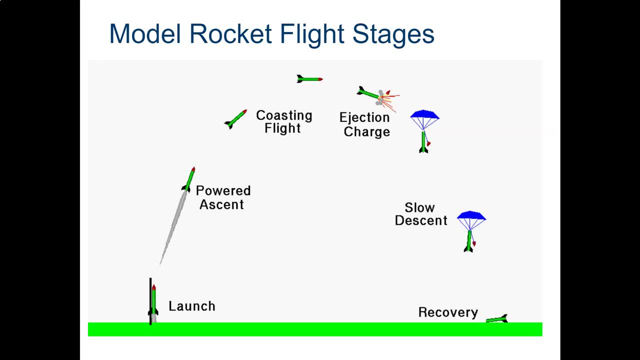 slide in just so you can see kind of what's coming up. but you should know that what each stage is. so when we launch, this is the powered part of the flight. so this is when the rocket engine is on, when it's thrusting, it's going to. 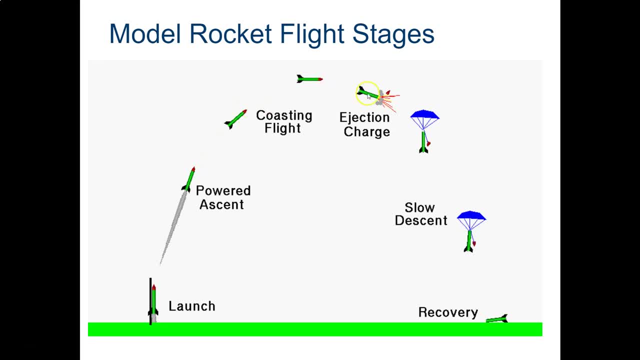 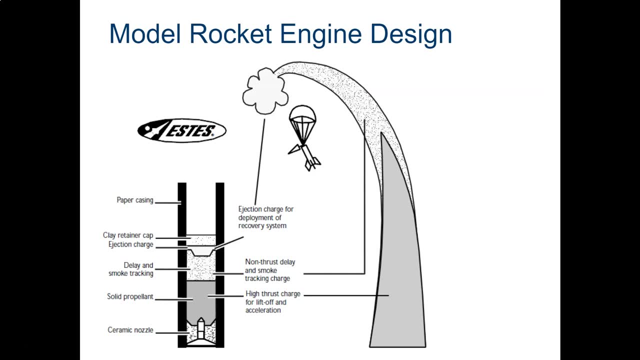 coast. after the engine cuts off, it's going to eject a charge and then come down. this is what a cross-section the model rocket engine looks like. it's a solid propellant, just like you can see here. so if we cut it in half and and took a look at it, this is what it would look like. so it has down at the 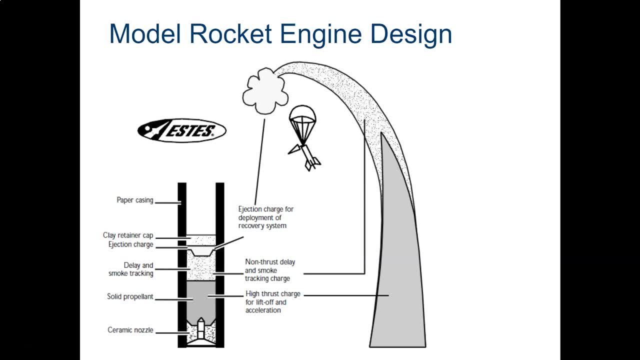 bottom and I'm not going to move my cursor a little bit down. at the bottom you see the nozzle and it expands, just like we would expect. it has a solid propellant and then it has a delay in it and then at the top here it has a little. 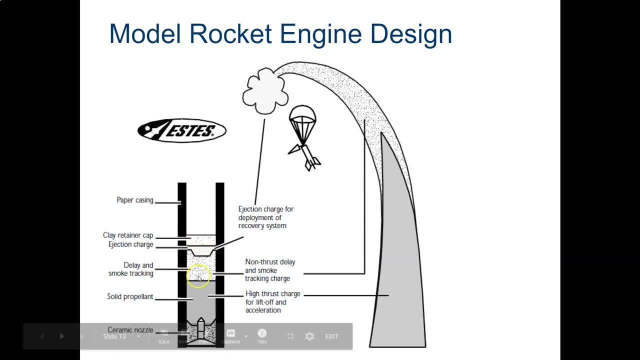 explosive charge, so that that is a propellant, but instead of blowing down or out, it actually blows up. so what happens is when the the flame reaches or the temperature, when this burns through and this part burns, it ejects the the parachute. so here's just a demonstration, if you will. 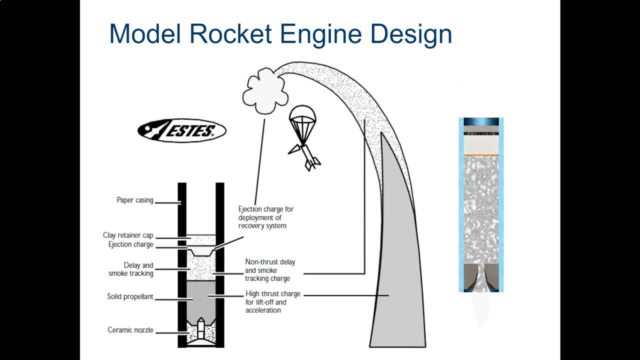 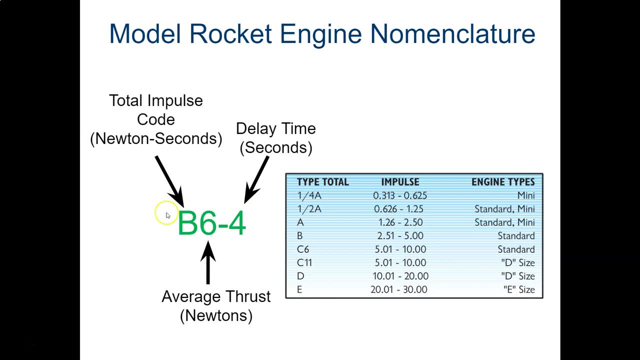 of what that looks like and real quickly, here's sort of the decoder ring- secret decoder ring to look at different types of model rocket engines. I'm not going to direct you here. I'm going to talk about this in the future, but for now just know that there's a code associated with total impulse. so 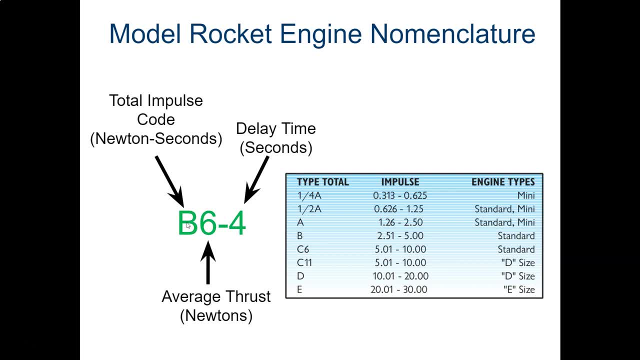 any letter that you go farther in the alphabet it is higher than the previous one. so B has more total impulse than a. C has more total impulse than B and usually that impulse doubles. so here you can see B has more total impulse than B, has a range of 2.5, 1 to 5, and we're going to find from Estes that it's 5 C. 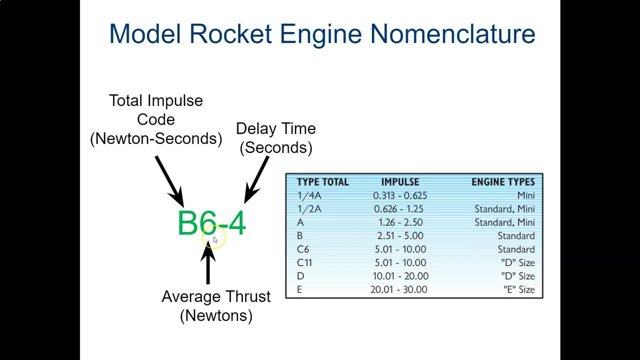 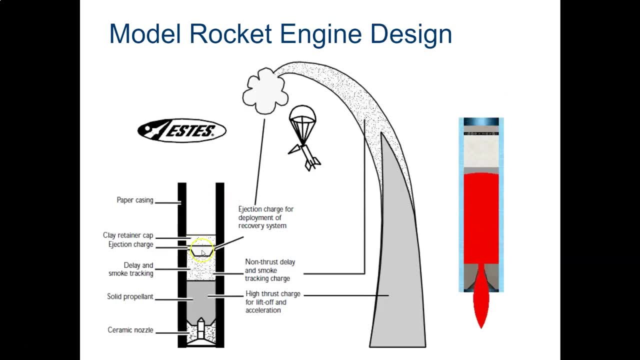 would be 10 and so on. so the next number indicates the average thrust and then the delay time goes back to the previous slide. that's how much time it's going to take from when the propellant stops burning and it's going to continue to burn through here for four seconds and then that charge is going to come out.